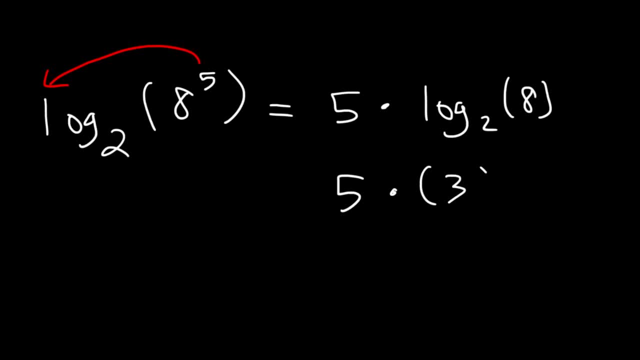 2 to the 3rd is 8, so log base 2 of 8 is 3.. And 5 times 3 is 15.. Now let's work on this example: Log base 2 of 16 times 8.. 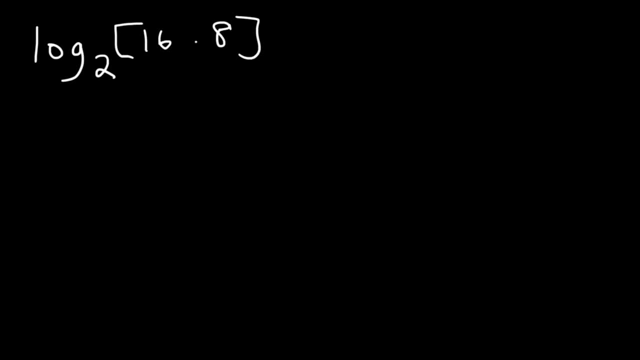 So we can use the product rule to separate the 16 and the 8.. If you recall, log of 8 times 8 is 8. So we can use the product rule to separate the 16 and the 8.. So we can use the product rule to separate the 16 and the 8.. 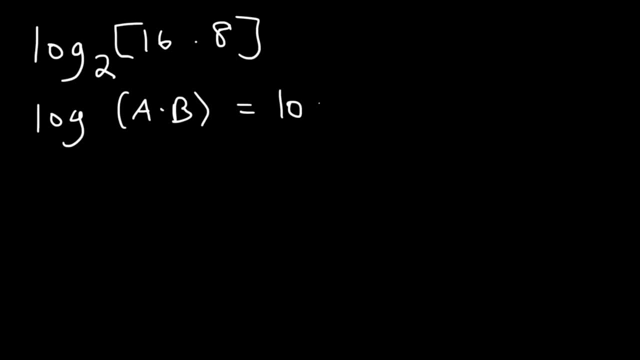 plus log base 2 of 8 x B is equal to log A plus log B. So therefore log base 2 of 16 times 8 is going to be log base 2 of 16 plus log base 2 of 8.. 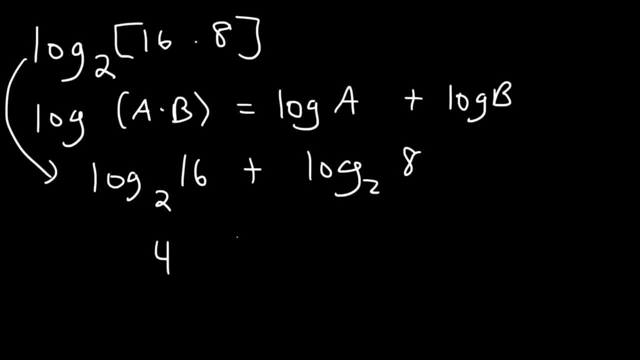 Now log base 2 of 16, that's 4, because 2 to the 4th power is 16.. Log base 2 of 8 is 3.. So the final answer is 4 plus 3, which is 7.. 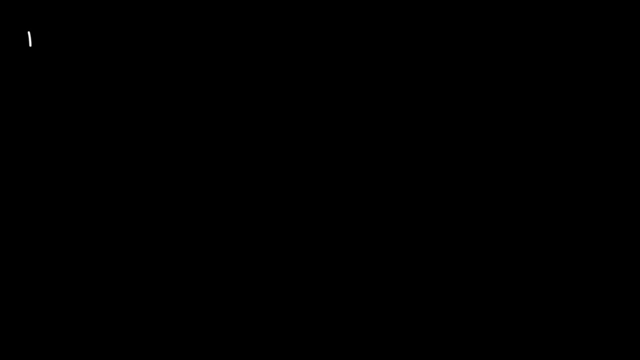 try this one: log base 3, 27 times 81, so first let's separate it into two logs. this is log base 3 of 27 plus log base 3 of 81. 3 to the third power is 27, so log base 3 of 27 is 3. 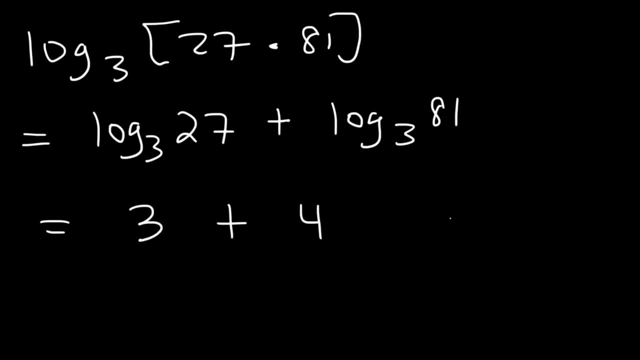 log base 3 of 81 is 4, because 3 to the fourth power is 81 and this adds to 7. now what about division? what is log base 4 of 256 minus 64? so, using the quotient rule, log a divided by b is equal to log a minus log B. so therefore, 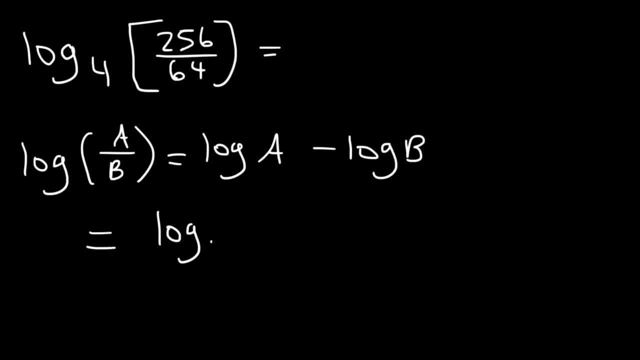 this is going to be log base 4 of 256, minus log base 4 of 64.. 4 to the 4th power is 256 and 4 to the 3rd power is 64, and 4 minus 3 is 1 and so 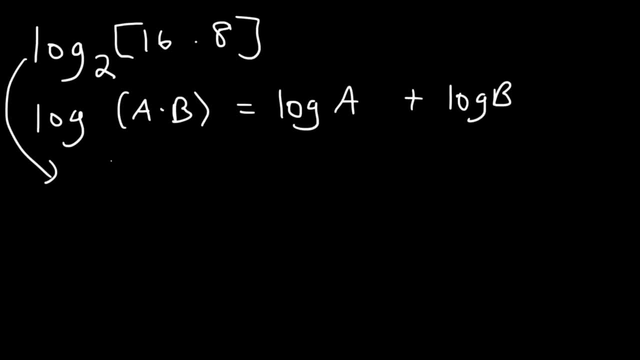 So therefore, log base 2 of 16 times 8 is going to be log base 2 of 16 plus log base 2 of 8.. Now log base 2 of 16, that's 4, because 2 to the 4th power is 16.. 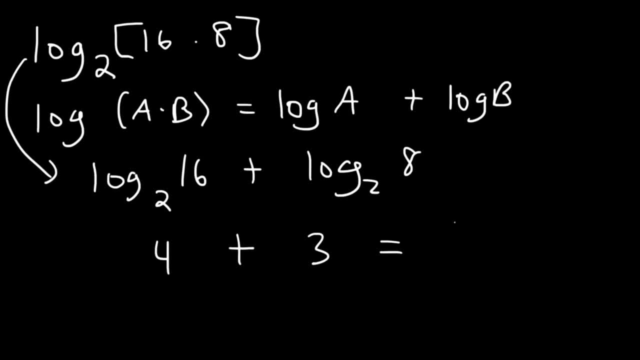 Log base 2 of 8 is 3.. So the final answer is 4 plus 3,, which is 7.. Try this one Log base 3, 27 times 81.. So first let's separate it into two logs. 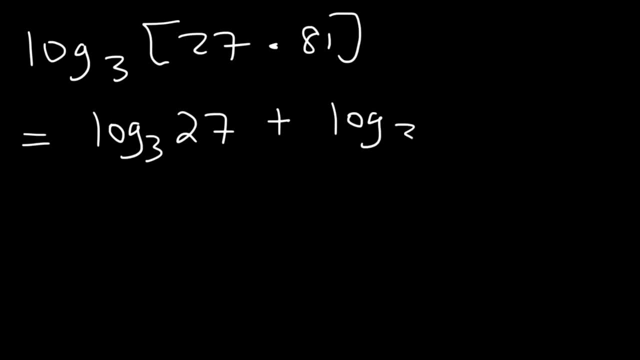 This is log base 3 of 27 plus log base 3 of 81.. 3 to the 3rd power is 27,, so log base 3 of 27 is 3.. Log base 3 of 81 is 4, because 3 to the 4th power is 81.. 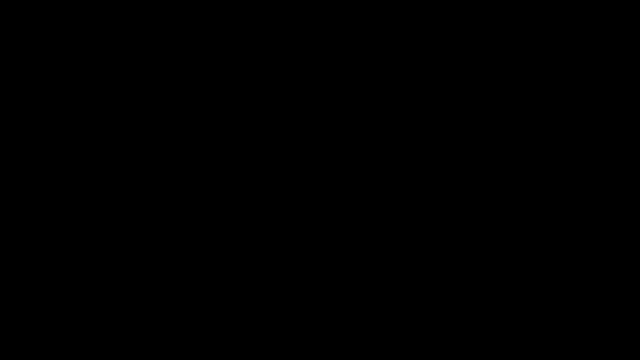 And this adds to 7.. Now, what about division? What is log base 4 of 256 minus 64?? So, using the quotient rule, log A divided by B is equal to log A minus log B. So therefore, this is going to be. 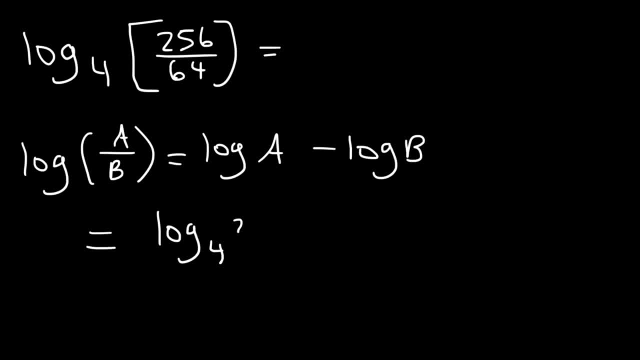 log base 4 of 256, minus log B Log base 4 of 64.. 4 to the 4th power is 256, and 4 to the 3rd power is 64. And 4 minus 3 is 1.. 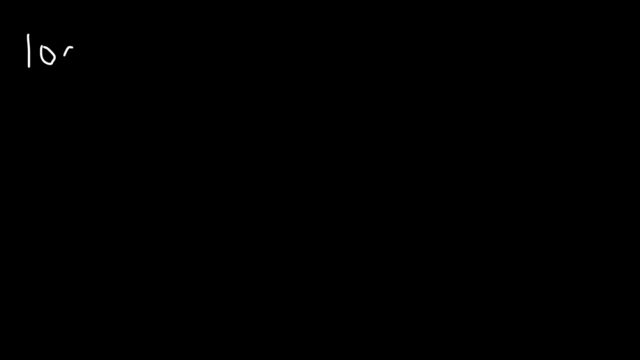 And so that's going to be the answer. Try this one: Log base 2 of 128 over 8.. So this is equal to log base 2 of 128, minus log base 2 of 8.. Now, 2 to the 7th power is 2.. 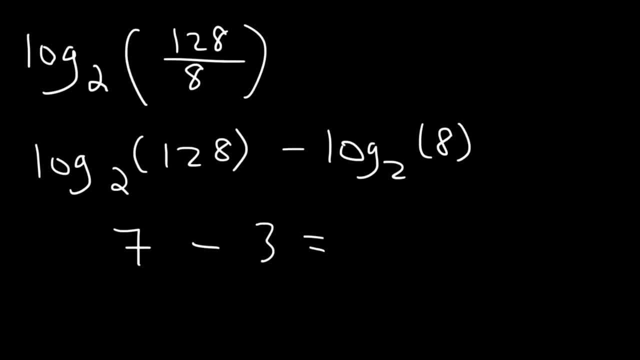 1 to the 7th power is 128, and 2 to the 3rd is 8.. So 7 minus 3 is 4.. And that's going to be the answer. Here's the last example: Log base 2 of 128 times 64, divided by 8 times 16, raised to the 5th power.